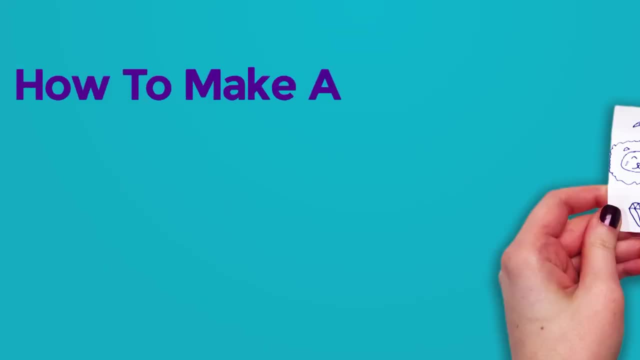 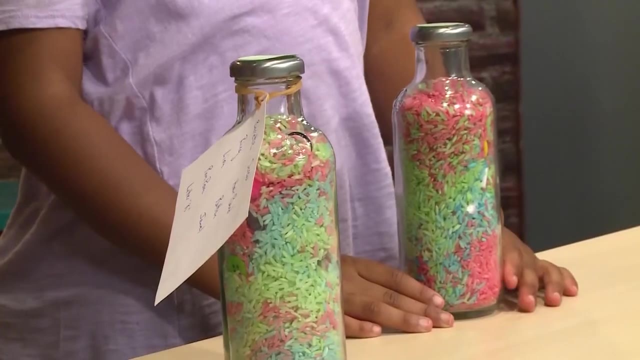 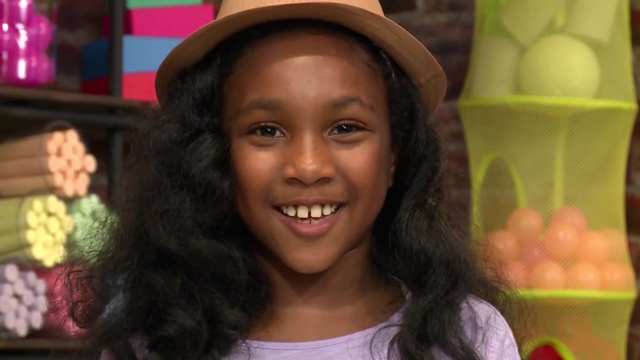 How to make an I Spy Bottle. Shhh, we're playing spies. We're making I Spy Bottles. What's an I Spy Bottle? It's a bottle where you spy things. We're going to show you how to make one, so you can play too. 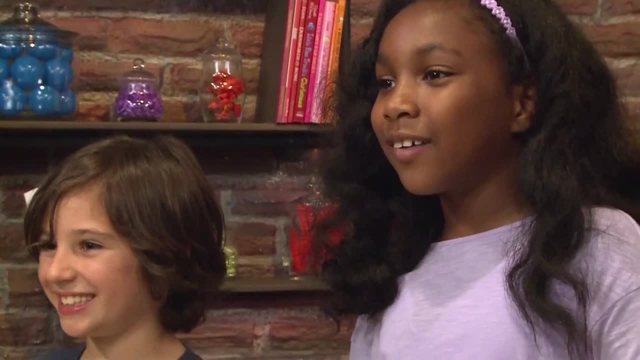 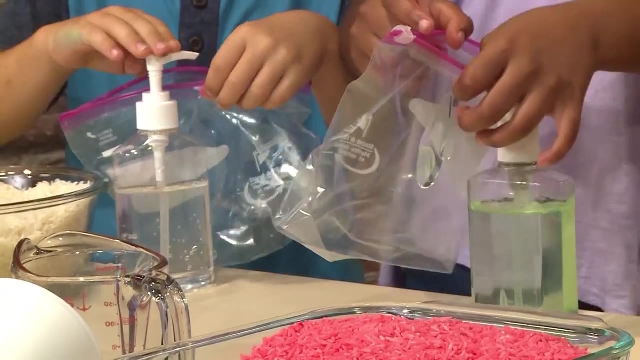 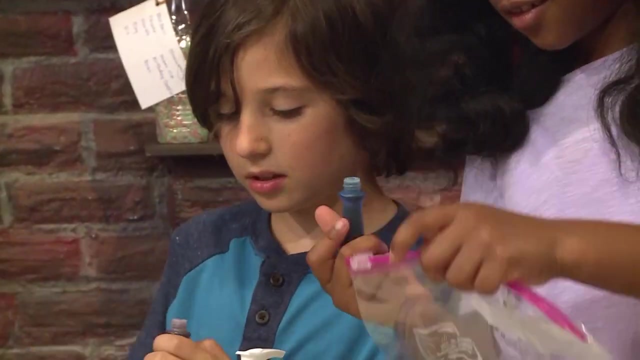 First, we're going to make colorful rice. You're going to first need a plastic bag. You put in four to five pumps of hand sanitizer- I want to make my rice red, I'm making mine's blue- Then put in four to five drops of food coloring. 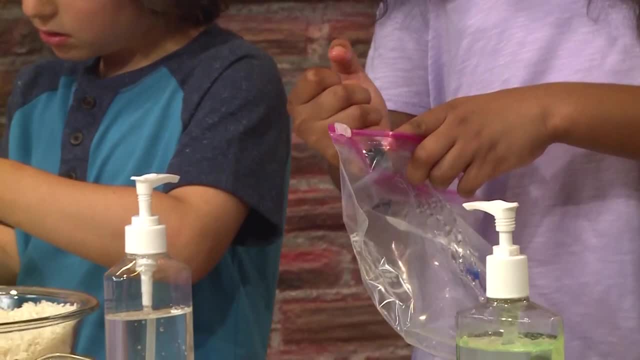 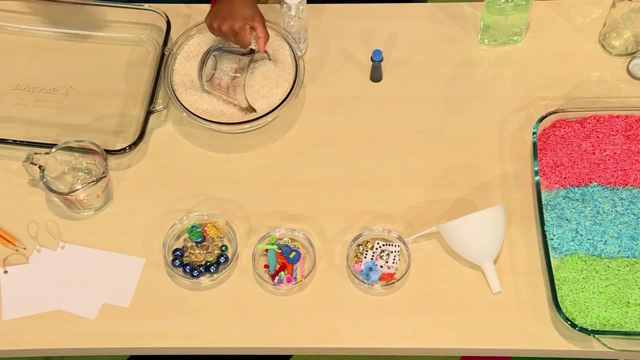 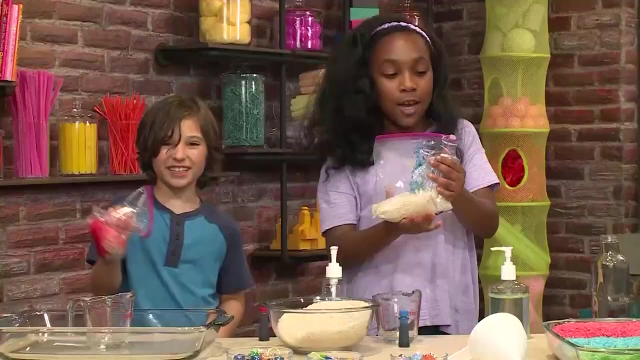 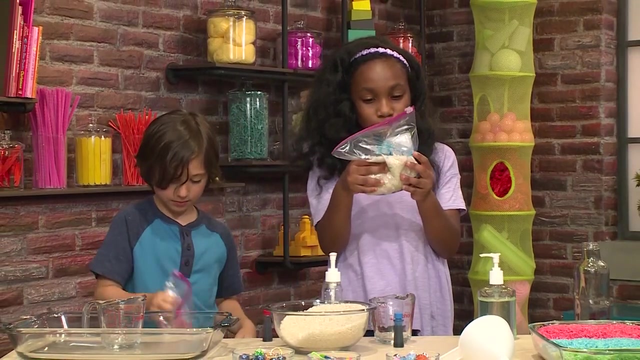 One, two, three, four, And then you're going to put a cup of rice And just put one cup. You need a spoon. You zip your bag And then you're going to put that rice and just swish it. 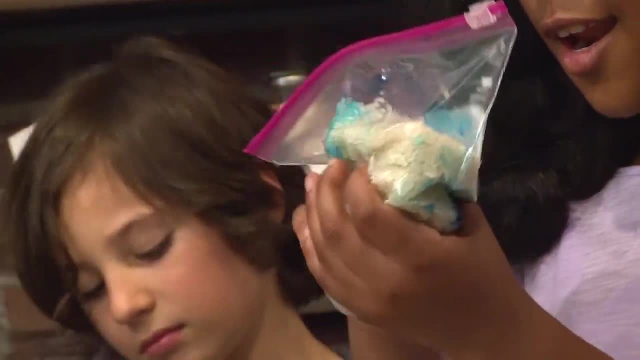 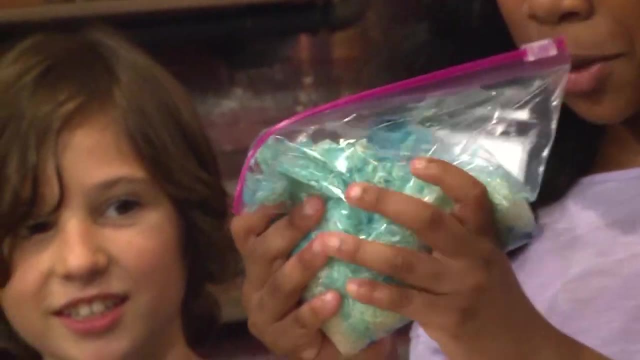 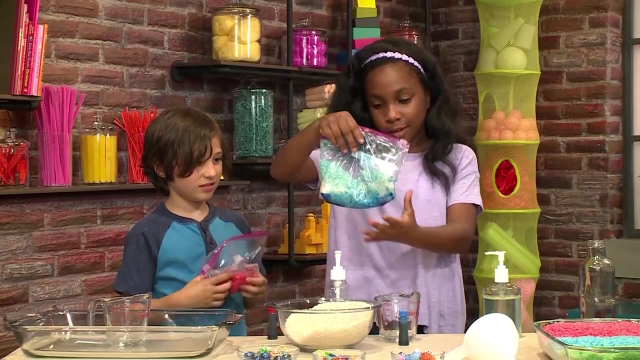 Just really nice. It feels so mushy, Mushy, mushy, mushy, mushy, mushy. Mine is all red, now Mine is blue, And then you need to dry your rice. It'll probably take an hour. 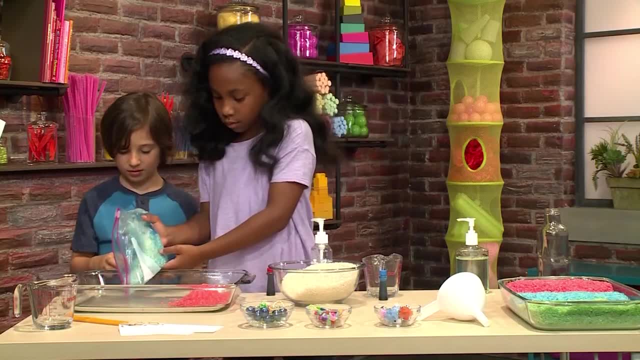 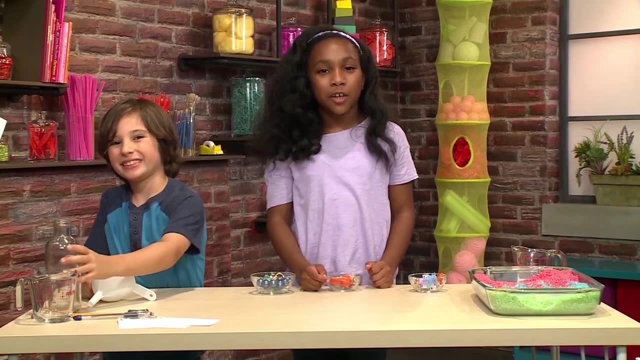 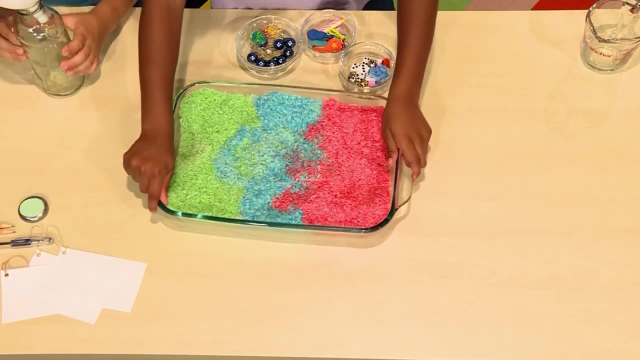 You could just pour it into a bowl. This is the rice that we made earlier, And now it's dry And now we're ready to make our I Spy Bottle. This bottle was old and recycled from sweet tea, So we're going to have a clear bottle, a funnel. 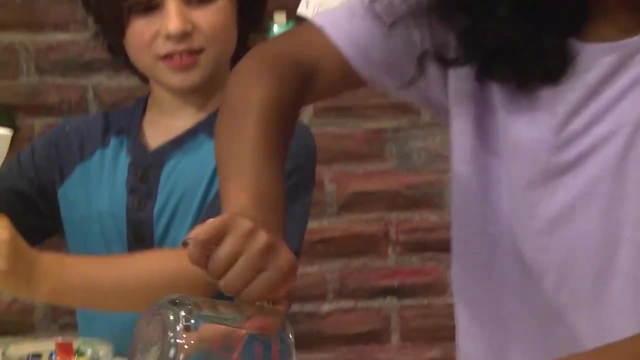 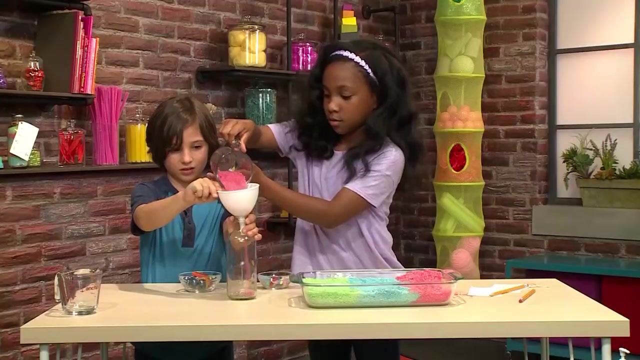 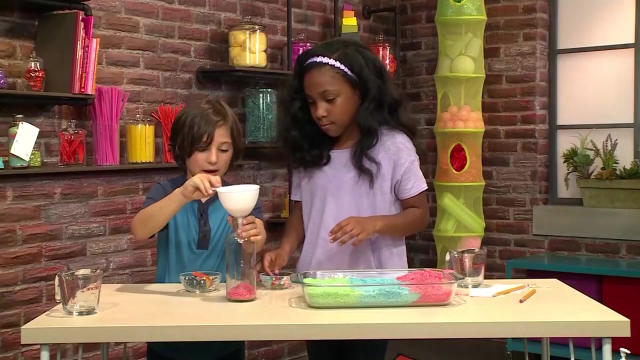 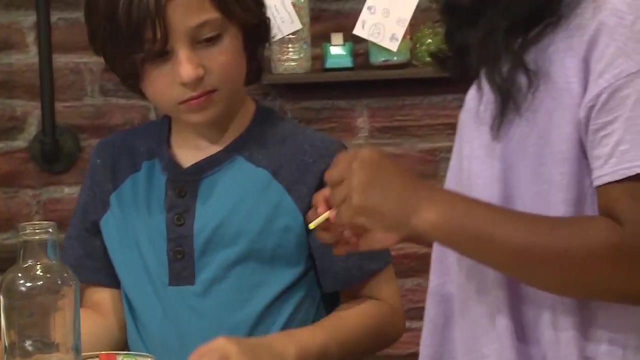 And here are some objects. So we're going to get a scoop In the red And the funnel makes the rice go through it, So then the rice will go into the bottle. Find some items to put inside the bottle. Here's some that we found. 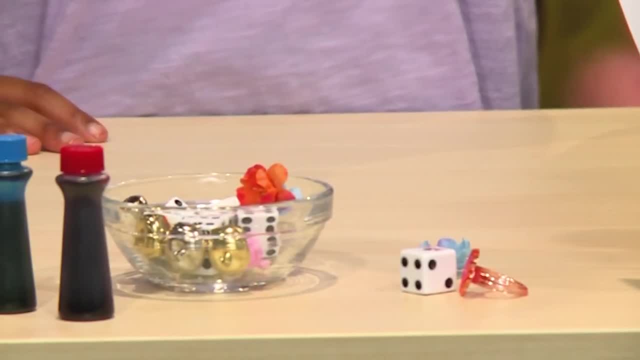 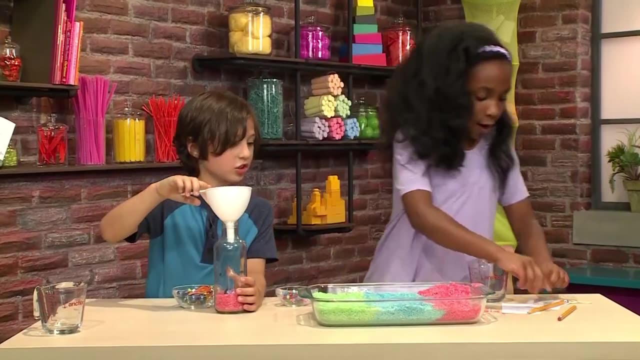 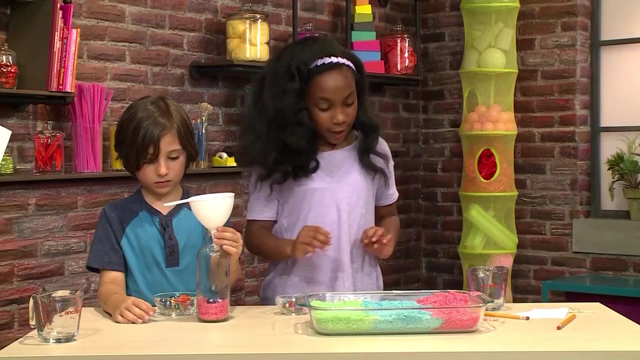 A paper clip, some candlesticks, some flowers. I added a blue ball. OK, And now we're going to write down what we just put on. We're going to write things down so we can find them later. So now we're going to get another scoop. 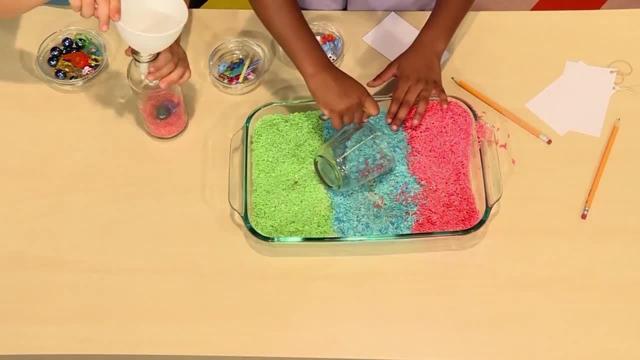 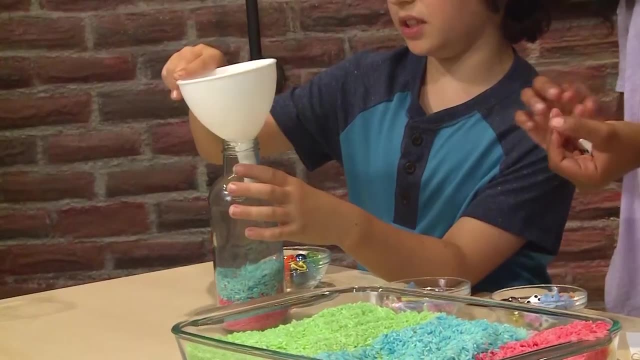 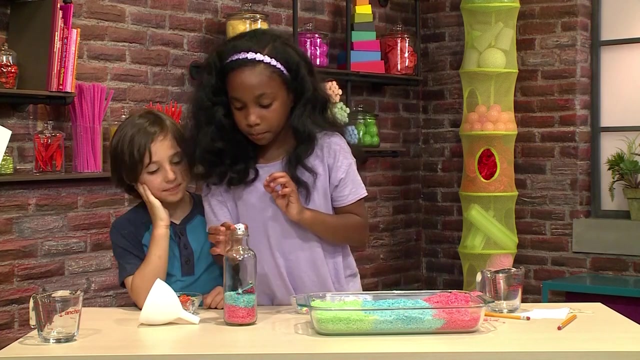 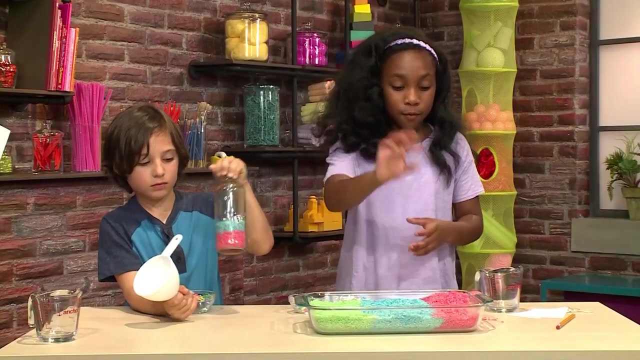 Now we're going to get the blue. This is going to be nice and colorful. So I'm going to put in the dice And he's just going to put in the skateboard. I'm going to put in like the red rice. 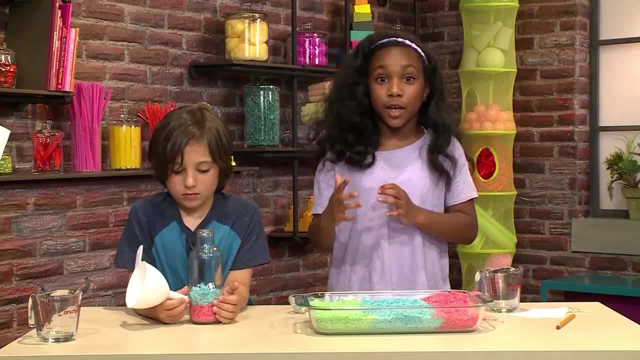 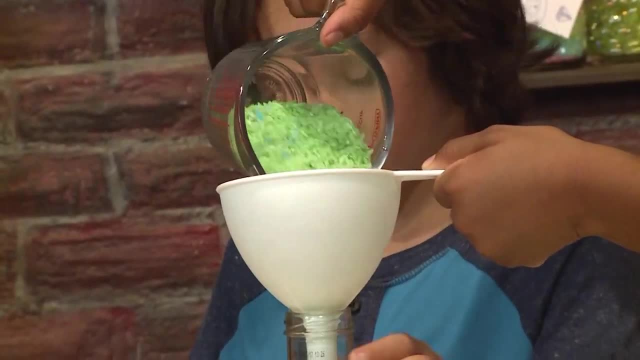 And then an object, And then the blue rice, And then an object, And then a green rice And an object, And I just repeat it and repeat it until it's full enough. OK, So now we're going to put in an object. 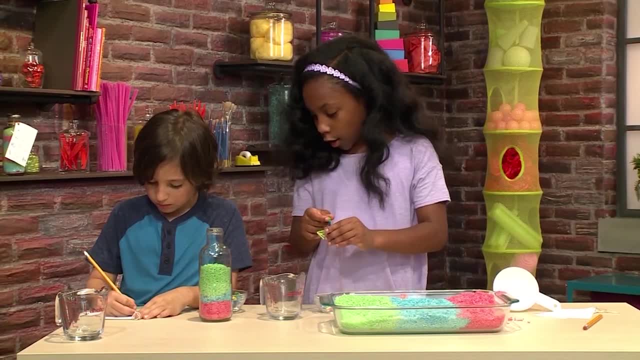 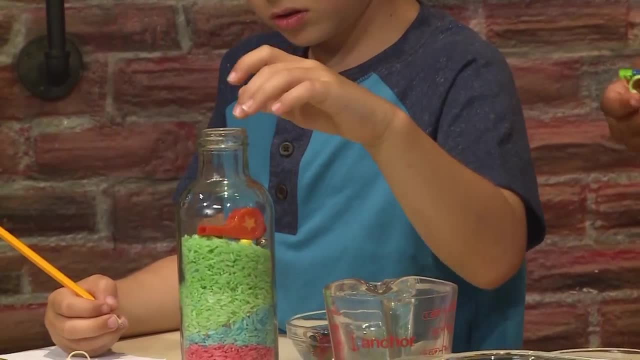 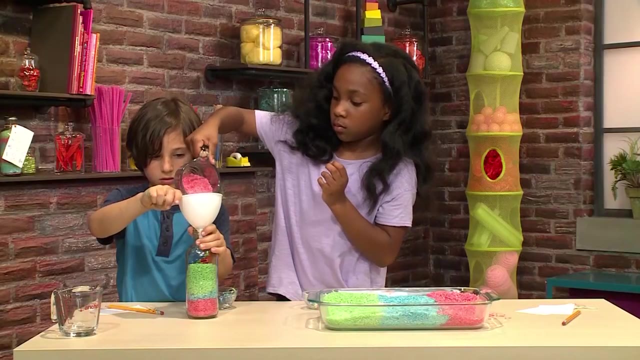 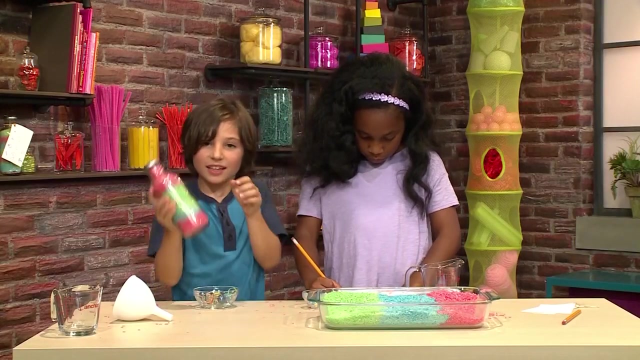 So I'm going to put in the guitar And Daniel's going to put in A whistle. The whistle, The whistle. OK, So now to finish our rainbow, Now I'm going to put the cap on And now I'm going to shake it up so I can find the objects. 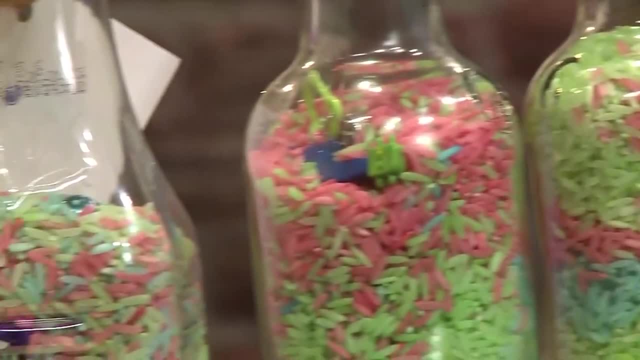 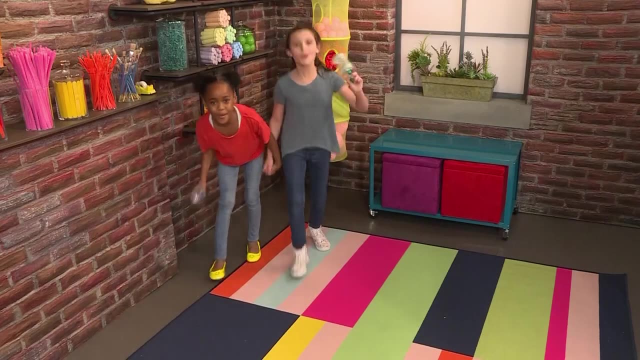 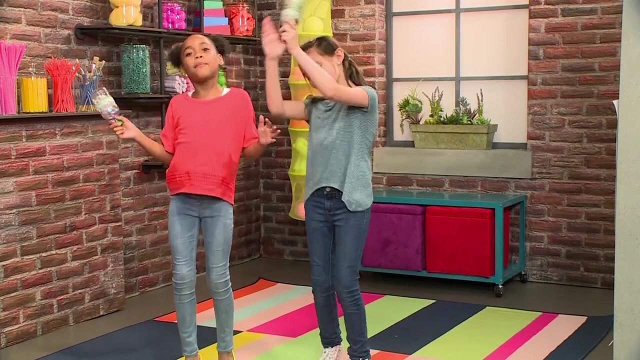 I found the guitar, And that's how you make an ice pie bottle. Shake it, shake it, shake it, Boom, boom, boom. We made shakers. Let us show you how to make one so you can play too. 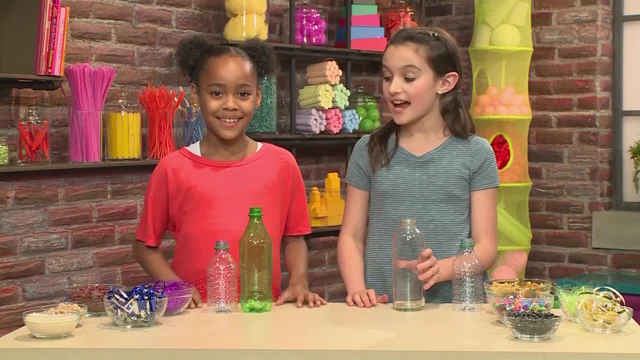 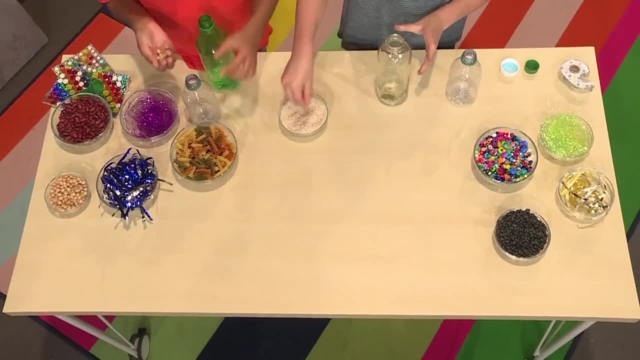 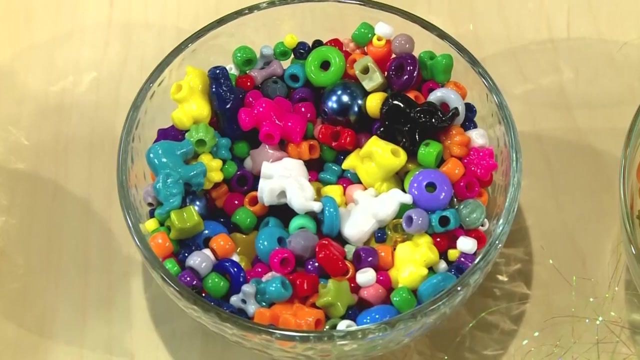 First, you need some recycled bottles. You can use glass or plastic, But make sure to clean out the bottle and it's all dry. Then you could fill your bottle with whatever you want. Different stuff will make different sounds. We have some beans, beads, rice and pasta. 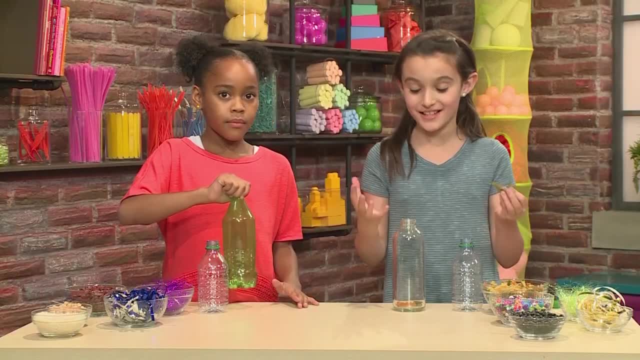 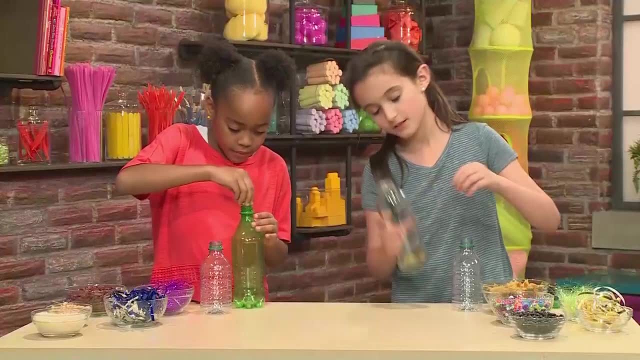 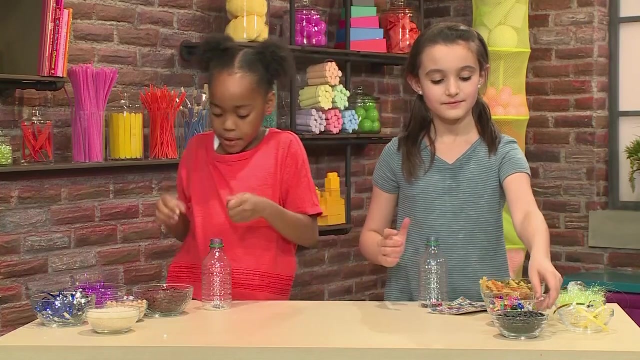 And I'm not going to put too much because I don't want such a heavy sound. Let's try this out. Ooh, that's nice. I like that a lot. I'm going to add some little beads so it doesn't make a boom, a boom, a boom. 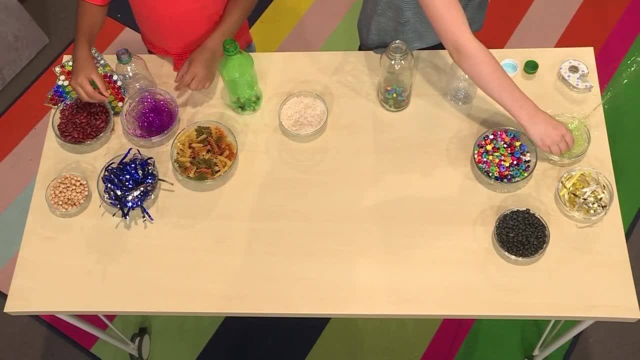 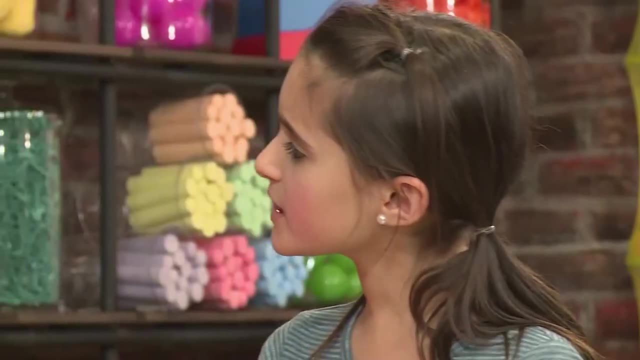 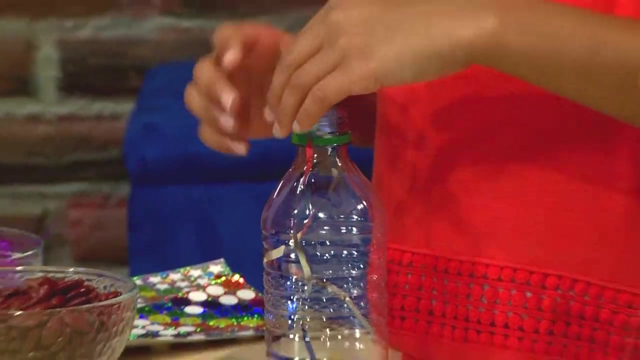 What I'm going to do is I'm going to put some. I'm going to put some of this nice pretty tinsel in the inside of my bottle. Do you think the tinsel will change the sound? Maybe I'm going to add some blue and silver ribbon. 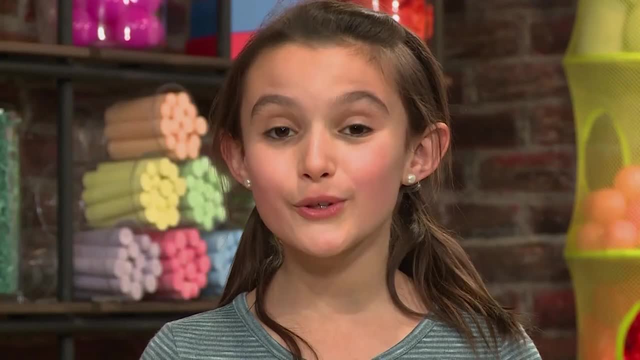 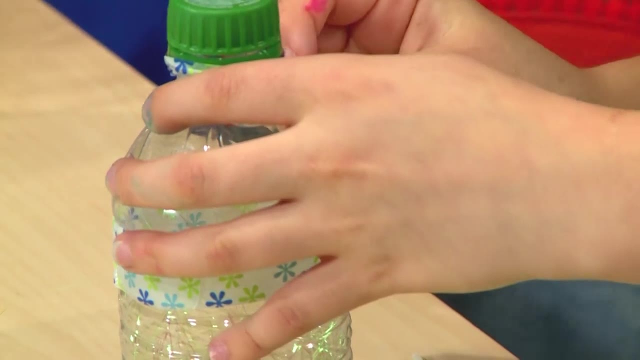 Big tip: Don't fill it up all the way to the top, because you want room for the things inside to shake, And then you put your cap on and seal it tight, And then you can decorate the outside too. I'm going to use some stars and smiley faces just to make it bling. 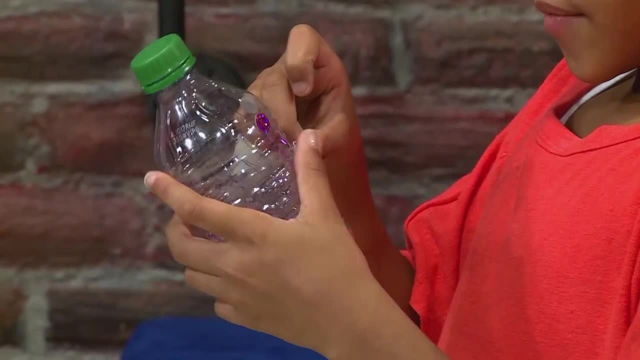 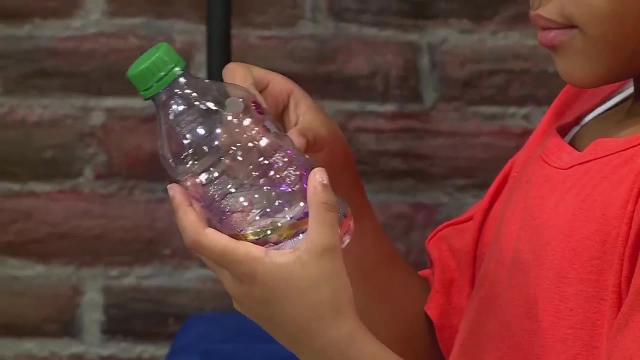 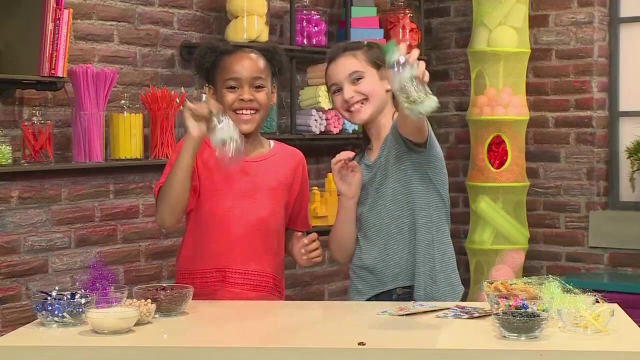 I'm going to use some of these star stickers. Yeah, these stickers are pretty. You can decorate it really any way you want. You can use ribbon, You could use duct tape, And that's how you make a shaker. How to make sand art. 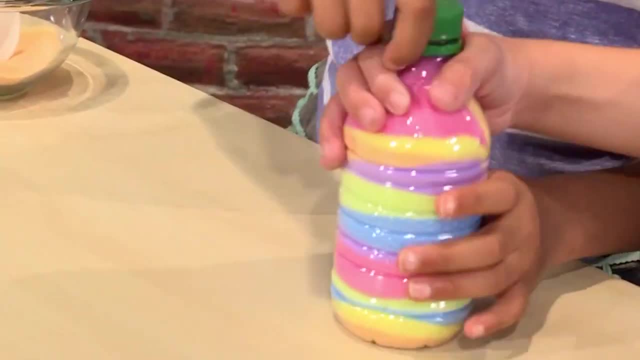 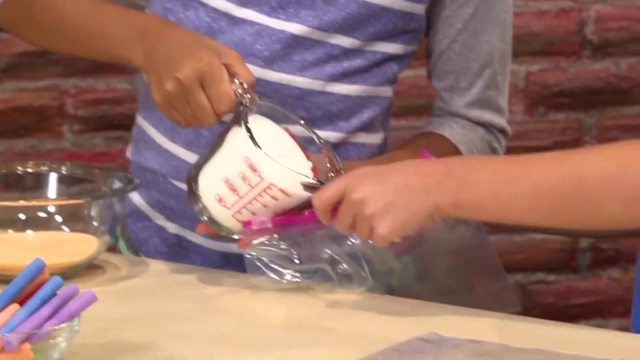 We're making beautiful sand art. today. We're going to show you how to do it, so you can play too. First, you need a plastic bag, a piece of sidewalk chalk and some salt. Pour about a cup of salt into your bag. 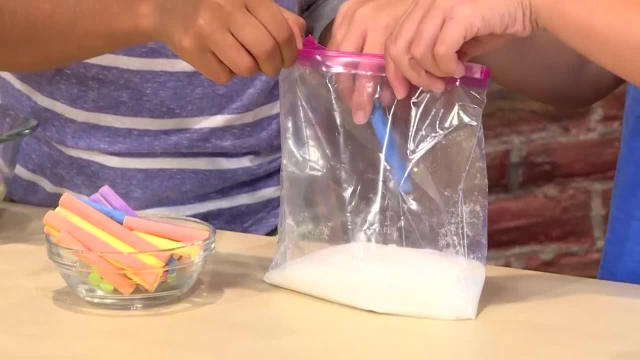 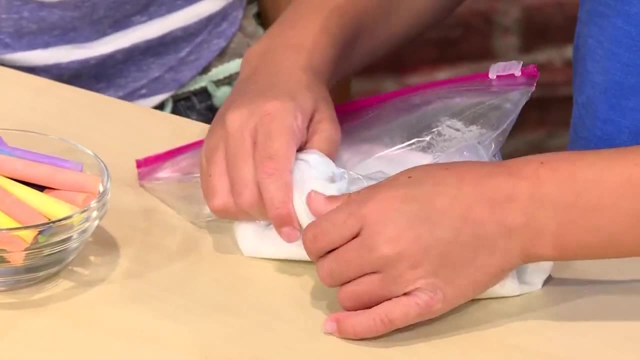 Now you'll need some chalk. Pick the color you want and put that piece of chalk in the bag too. Then you zip it back up and then rub, Rub the salt and chalk together. The salt is scratchy on the chalk. It causes the chalk to break apart in teeny tiny pieces. 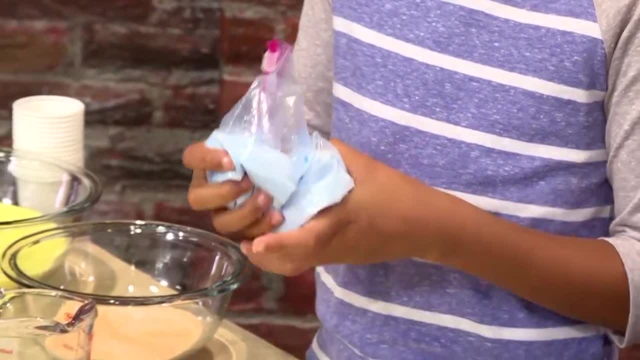 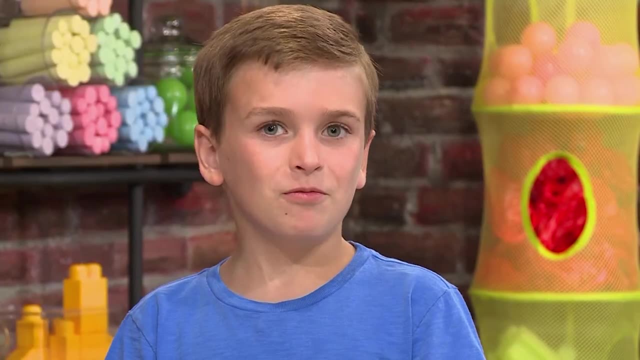 Those little pieces, mixed with the salt, becomes your sand. The more you rub, the darker the color of the sand would be. Once the salt is the color you want, you can pour it into a bowl. These are some sands we made earlier and we're going to show you how to pour it. 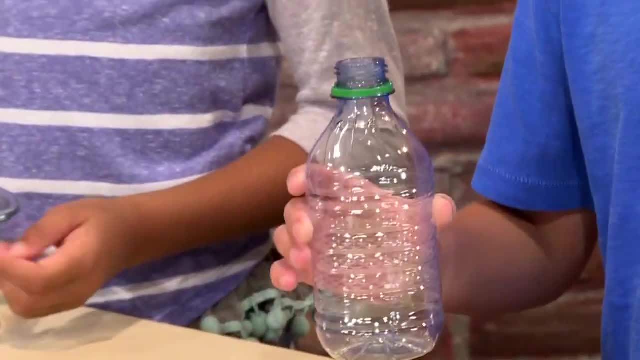 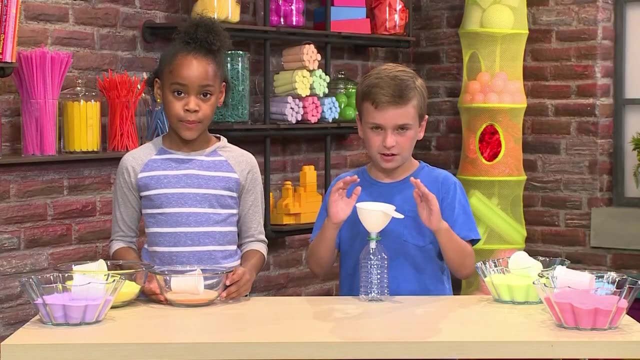 First, you'll need a recycled water bottle. It can be glass or plastic. Next, you'll need a funnel. You put the funnel on the top of the water bottle so you can pour the sand into the funnel And it comes into the water bottle. 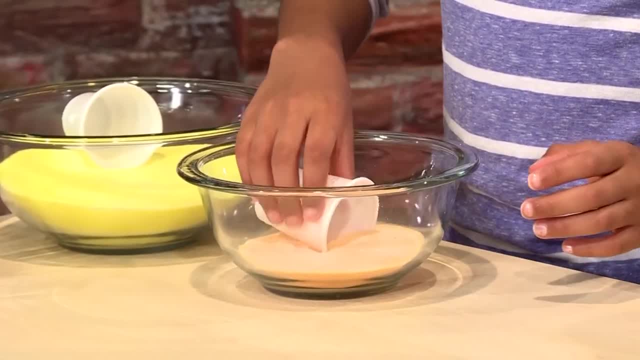 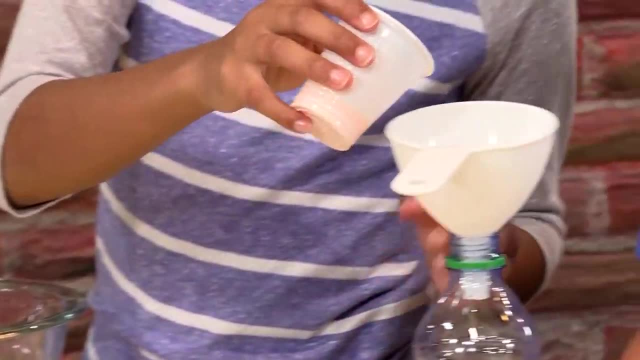 Now you're going to need some small cups to scoop the sand up. You need about a half of these little cups. You can choose whatever color you want. You can do it in a pattern or you can make it random. My turn. 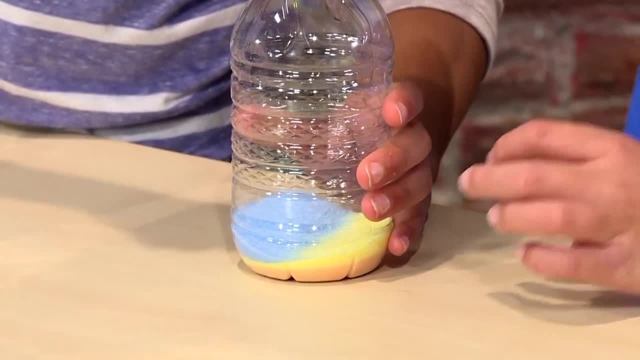 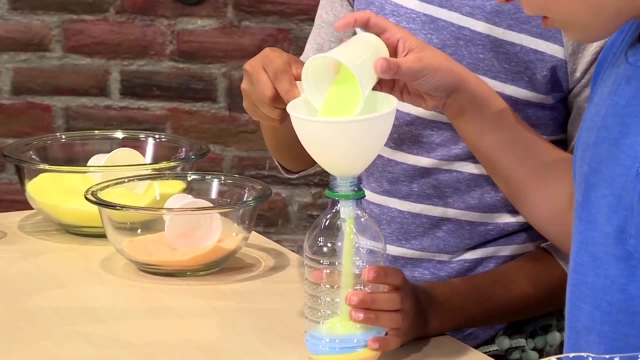 Now I'm adding blue. I'm going to add a little bit more blue because I want it to make a whole layer. Now I'm going to put some green in. Last but not least, some pink. I'll fill about half a cup of it. 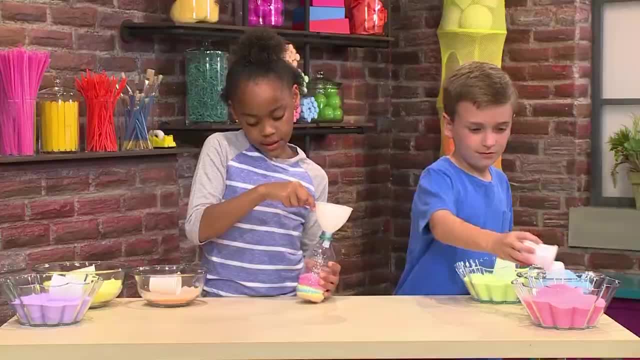 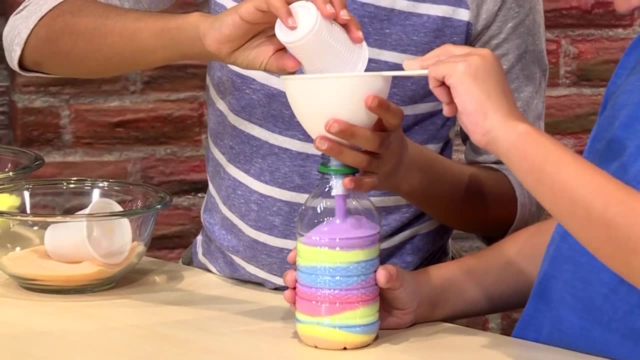 I'm adding a little bit more so it looks better. Now I'm going to tilt it to make it even. You just keep on layering the colors you want And then at the end you'll have a colorful sand masterpiece. There we go. 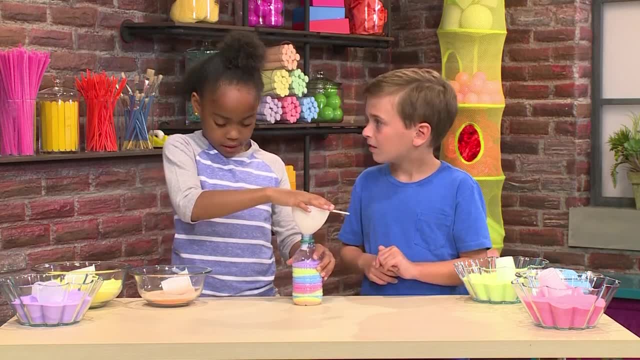 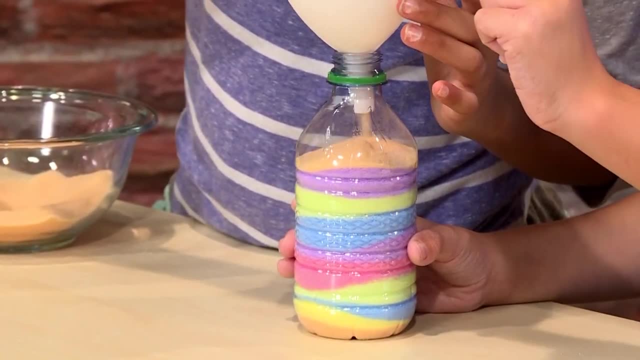 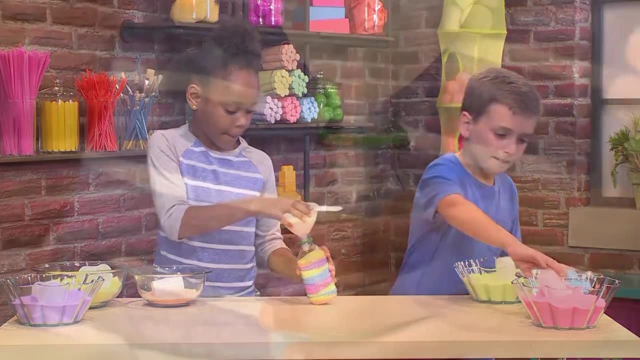 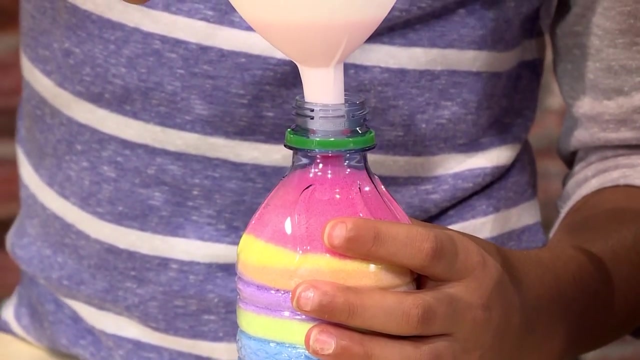 We'll just shake it a little bit to make it a little even. Can we add a little bit more orange? Yeah, Why don't we add some pink? Okay, This is about to be full. Now you need to put the cap on. 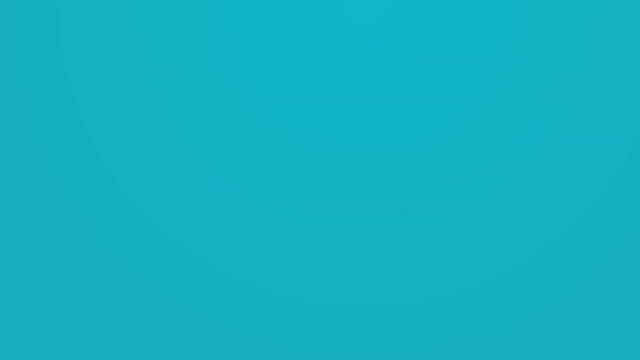 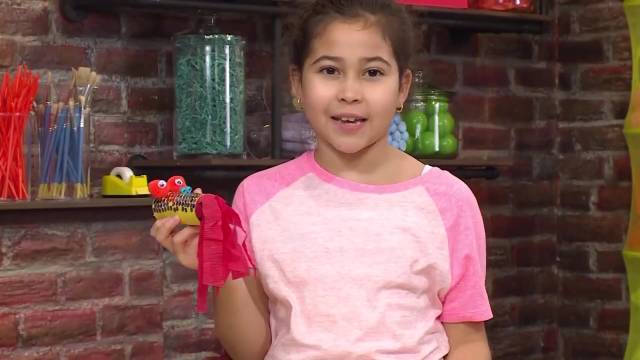 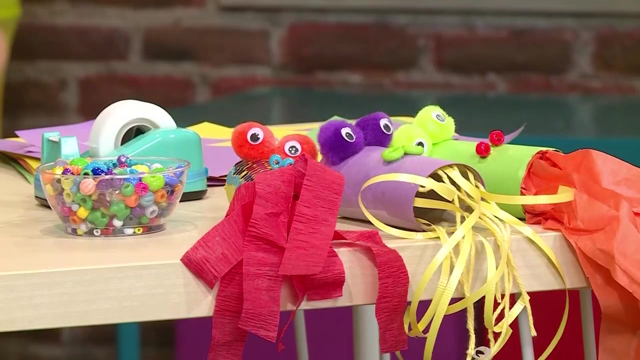 And that's how you make our masterpiece of sand art: How to make a fire-breathing dragon. This is my fire-breathing dragon. I named him Flame. Let me show you how to make one so you can play too. The first step into making a fire-breathing dragon is to get an empty toilet paper roll. 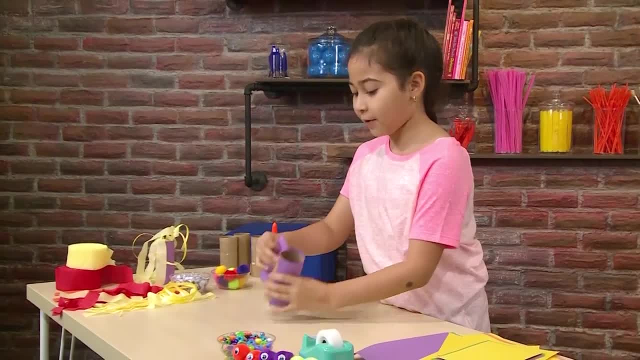 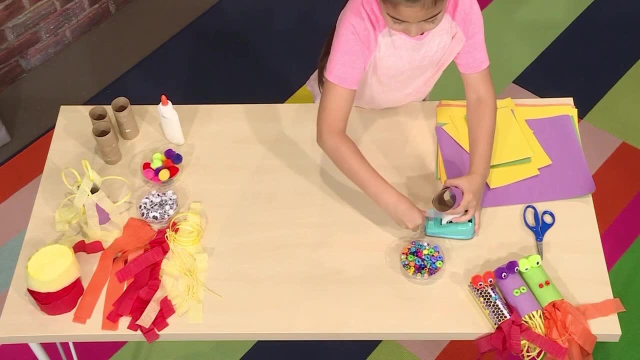 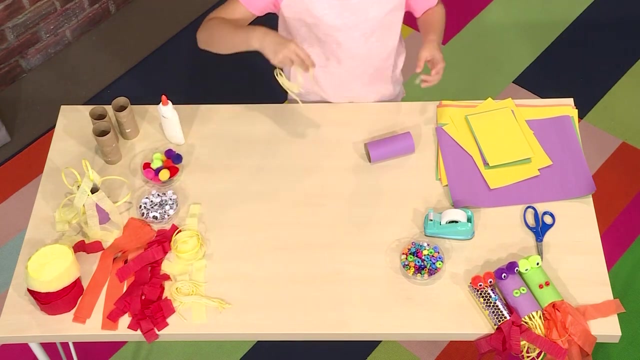 After you've gotten that, you get some construction paper and you wrap it around like this, Any color you want, And then you get a little tape and tape it, Then add the flames, You get some ribbons of your choice And you tape them to the inside of your dragon. 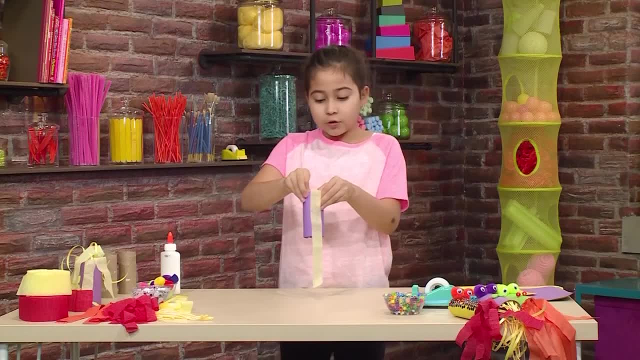 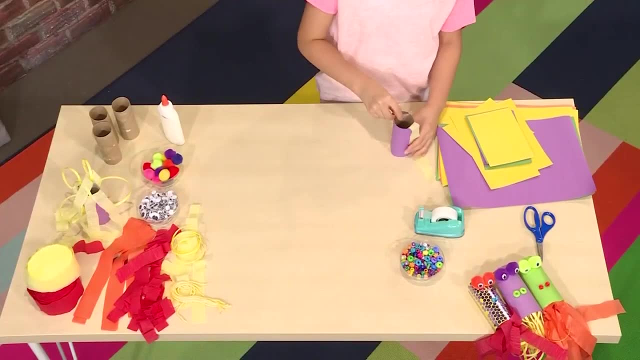 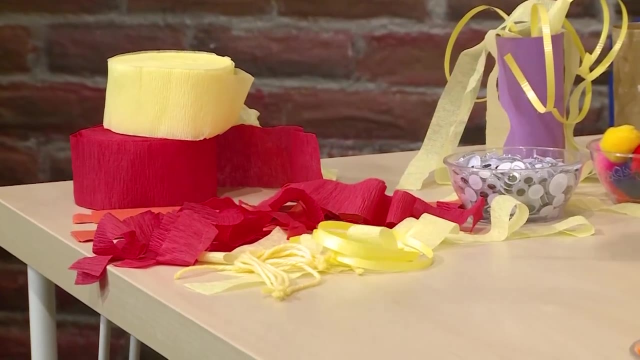 Here's a tip: If you want your dragon to blow out more fire, stick more to the top than to the bottom. You can use anything you want, including ribbons, yarn, other types of streamers. Put them in any way you want. 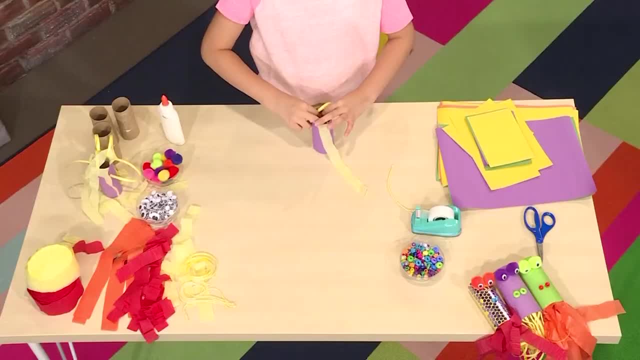 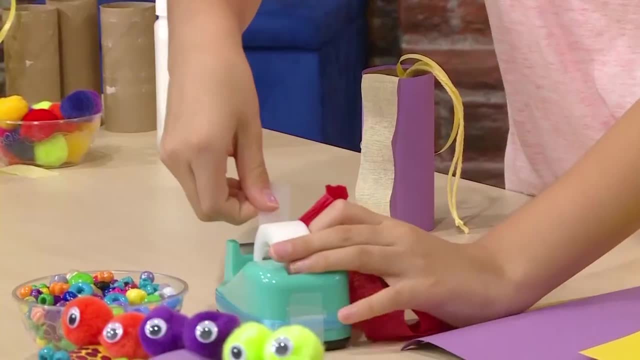 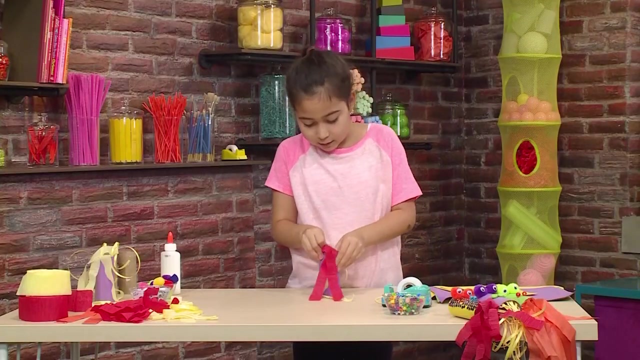 You can put some in the bottom, put some on the top. You can change the color, You can cut some paper out. You can really do anything you want with this dragon. I'm going to put different colors of streamers in and make it look cool. 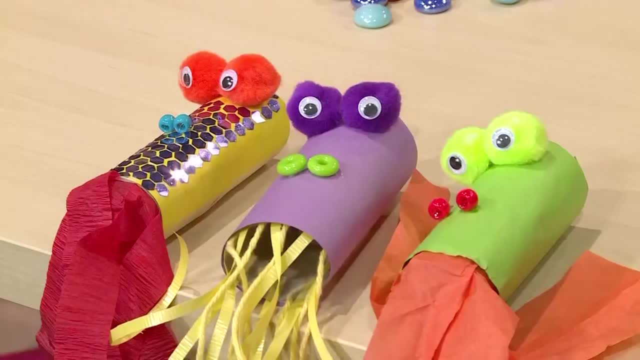 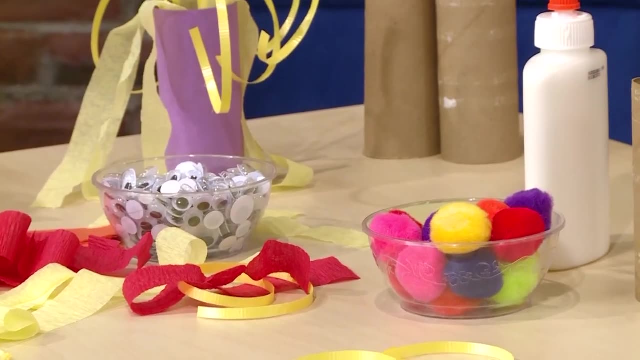 After this you can decorate it any way you want. Here are some I made earlier. You can add glitter or any kind of decoration. Then you can add a face. I'm going to put some pom-poms that are blue and green. 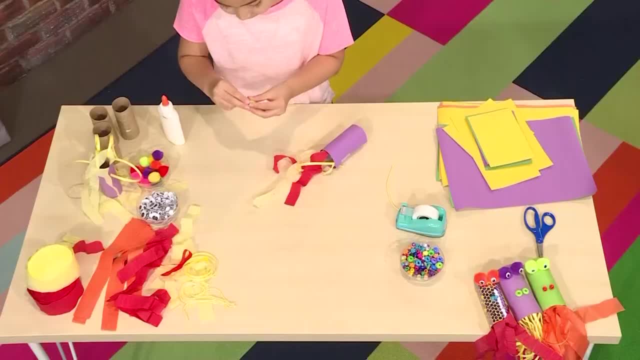 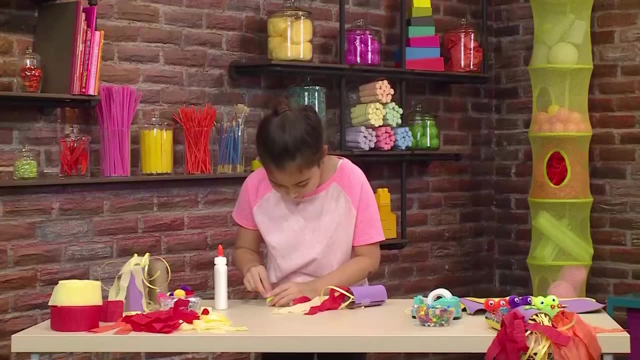 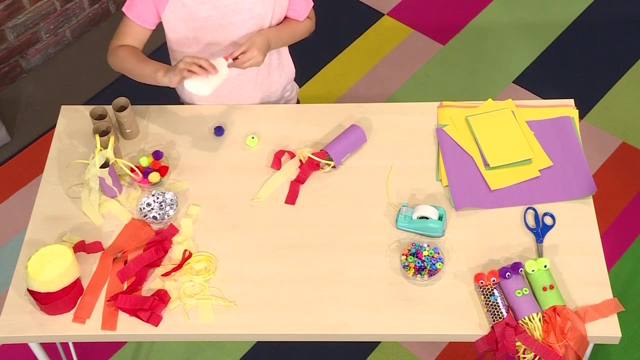 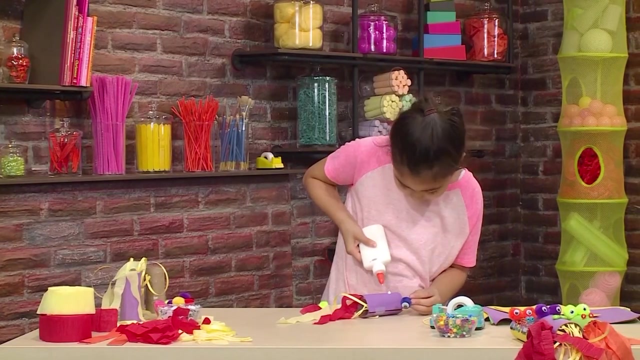 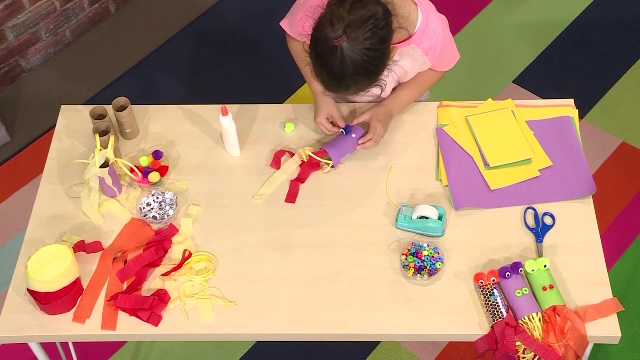 I'm going to put some googly eyes on them. Remember, you can do anything you want with this. You can attach them with glue, which is probably better for the pom-poms. Sometimes it's easier to put the glue on the toilet paper roll. 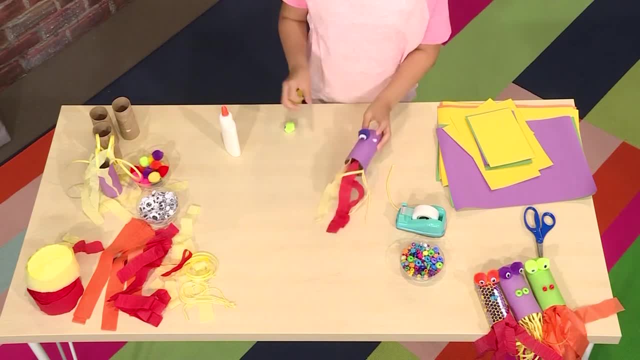 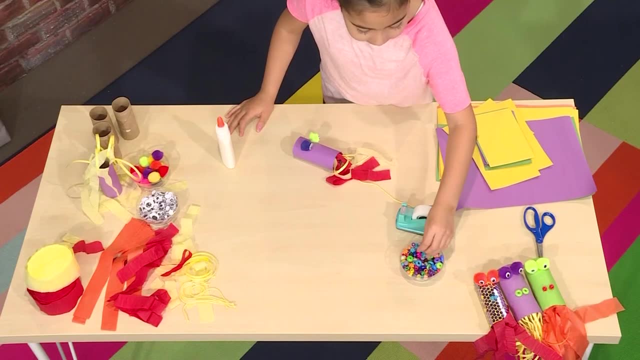 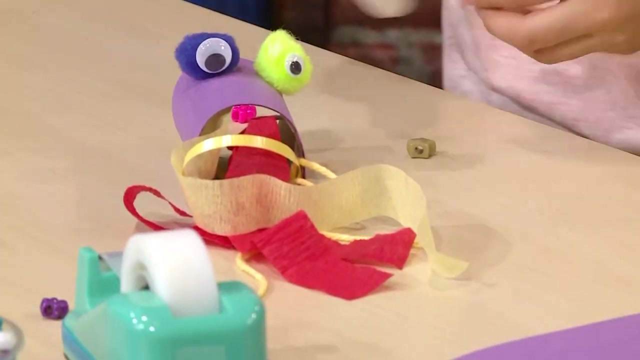 than putting the glue on the pom-poms, Then you need to add two little things for his nose. You can use beads, coffee beans, smaller pom-poms or buttons or whatever. Whatever you want, And I'm going to put some glue on the bead first. 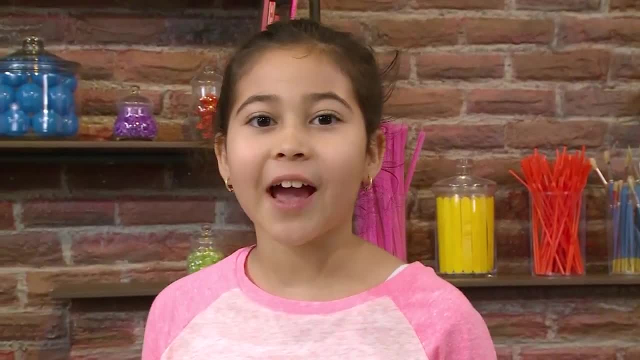 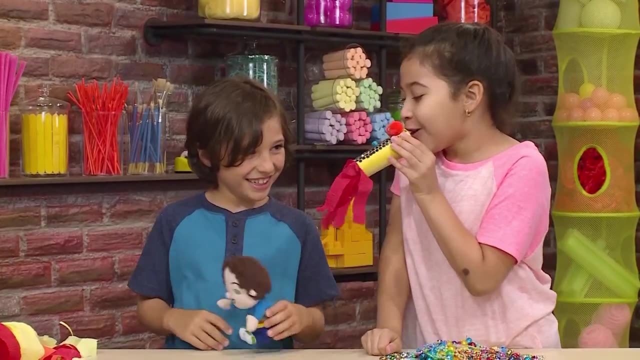 Wait for the glue to dry, And that's how you make your fire-breathing. dragon, Dragon, dragon, I want your jewel. No way, mister, Go away. No, no, no. Well then, can you at least touch my marshmallow? 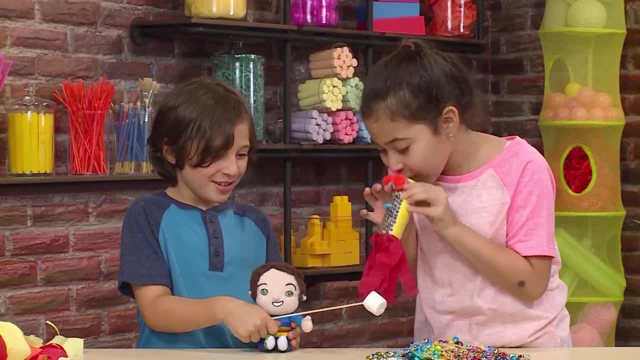 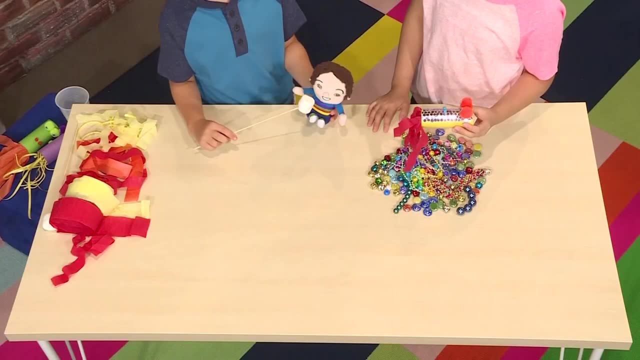 Sure, if that's what you want. Thank you, Yummy, yummy. Would you like a bite? Sure, It's so yummy. Yes, it is. I love marshmallows, but I love my jewels more. But you can have the rest. 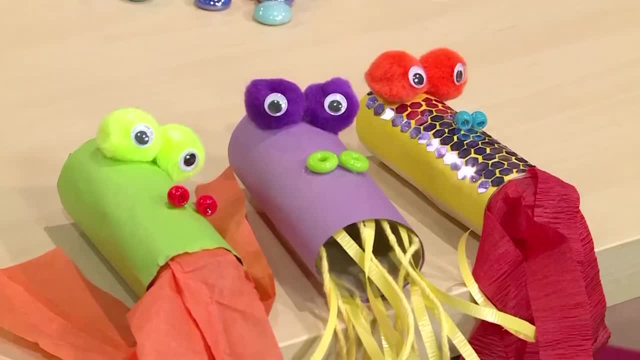 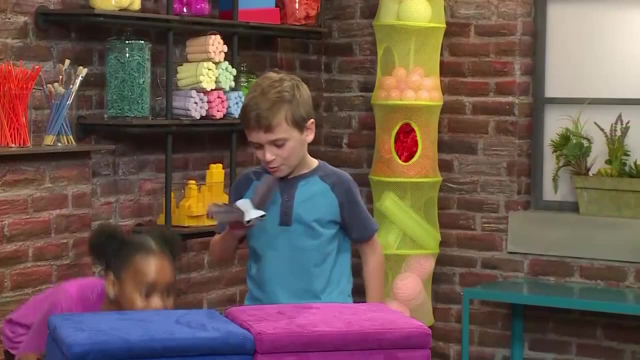 Thank you. Nom, nom, nom, nom, nom, nom. How to make a Halloween bat Boo, I'm so excited to go trick-or-treating- Me too, Mama, Mama, I want to go trick-or-treating. 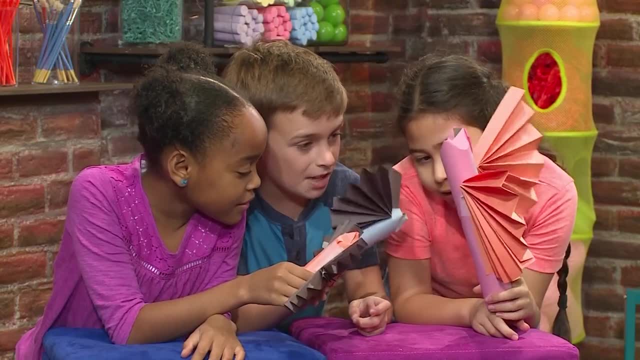 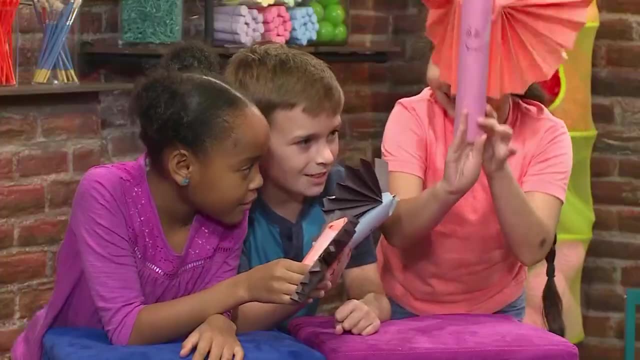 I'm not sure, Yeah, but the moon is out, It's full And the ghosts are out. It's the perfect Halloween day. Okay, Well, only because it's Halloween, Woohoo, Let's go Wee. 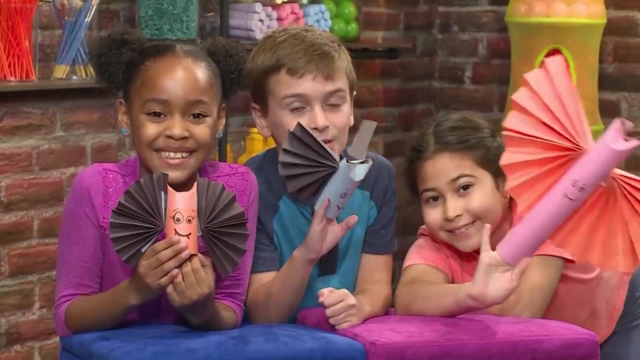 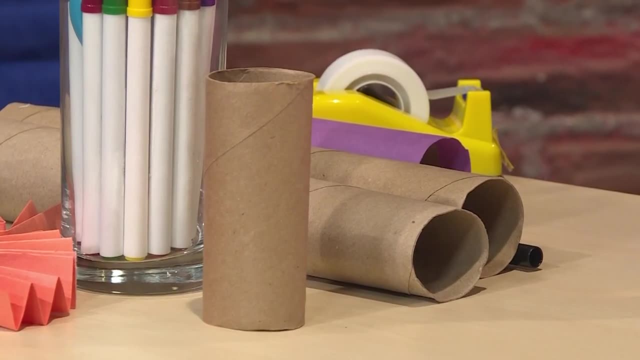 We made our own Halloween bats. We're going to show you how to make one so you can play too. Here's how you make a Halloween bat. First, you need toilet paper tubes. Then you'll need some paper of any color. You want the paper to be about the size of your toilet paper tubes. 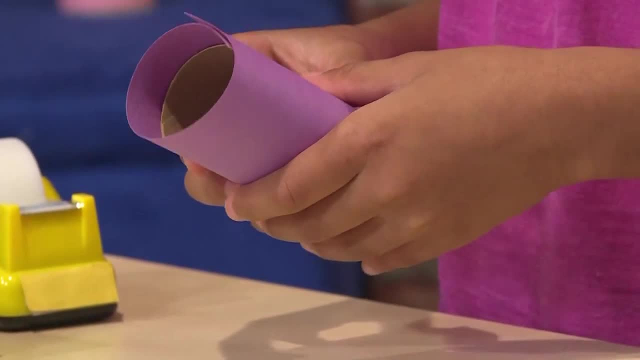 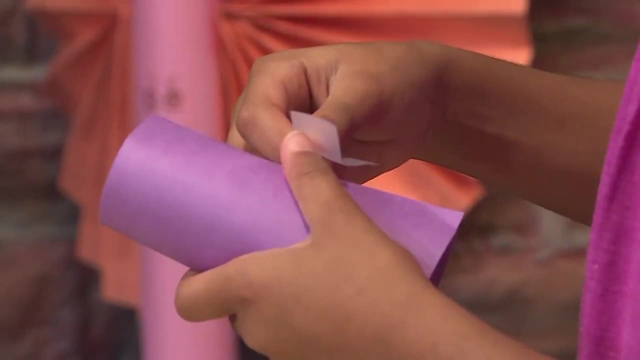 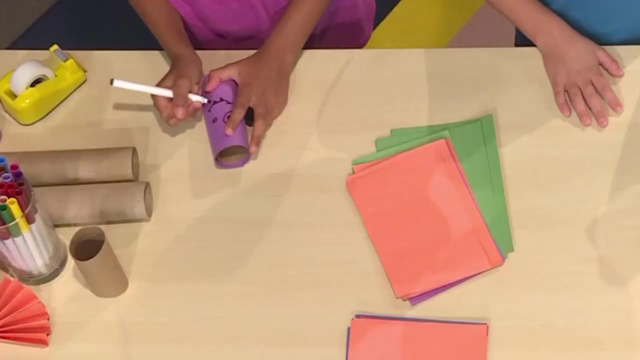 You're going to wrap it around the bat, Wrap the paper around the toilet paper tube. Then you're going to tape the edges of the paper together so it will stay wrapped around. Then you're going to draw on your face. I'm going to draw eyes, fangs and a mouth. 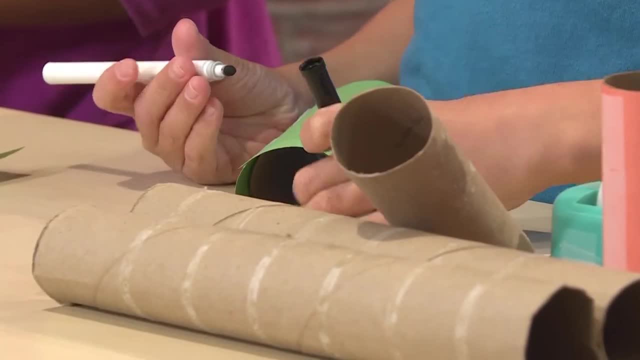 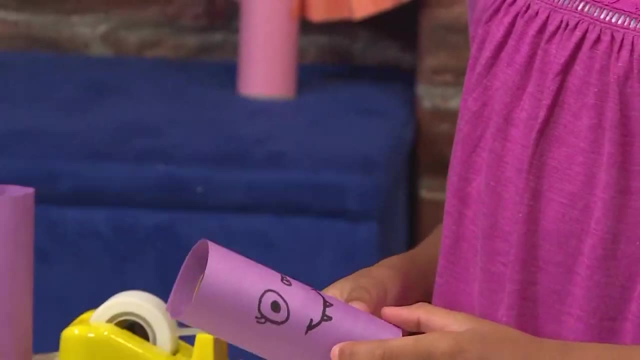 I'm going to draw eyes and just fangs. There I made the face for the bat. Don't put your face too close to the top, because you're going to need space for the ears. The next step is to add your wings. 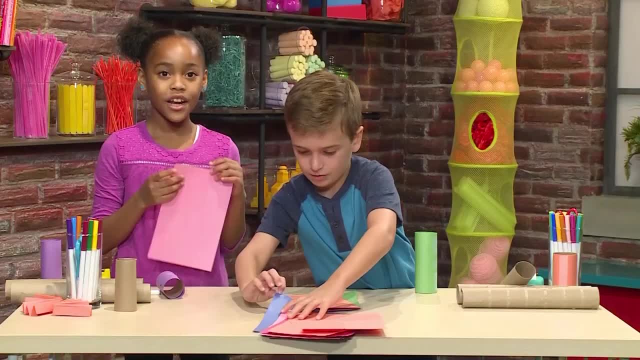 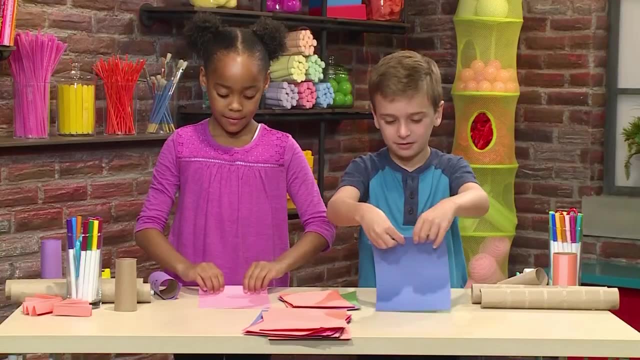 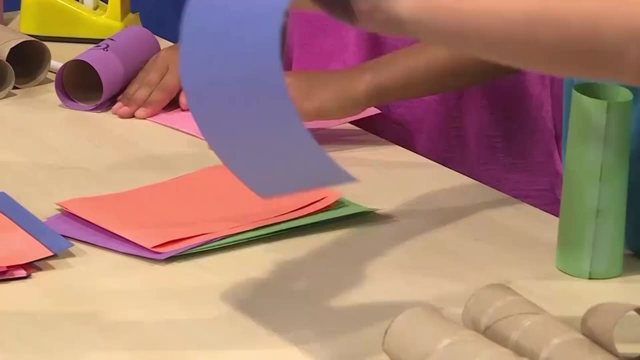 You're going to need another piece of paper. Then you're going to kind of make a fan. You're going to fold on one side and then fold on the other, And then just keep doing that, Just keep folding back and forth until you get a fan. 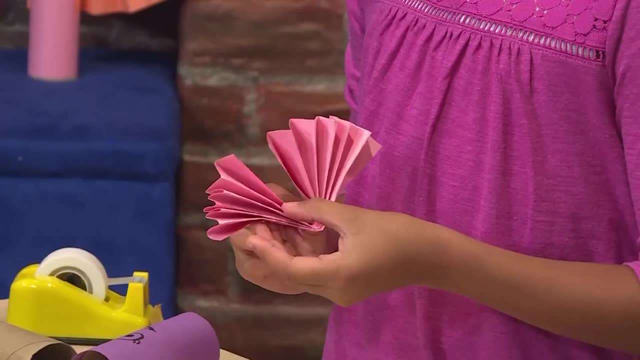 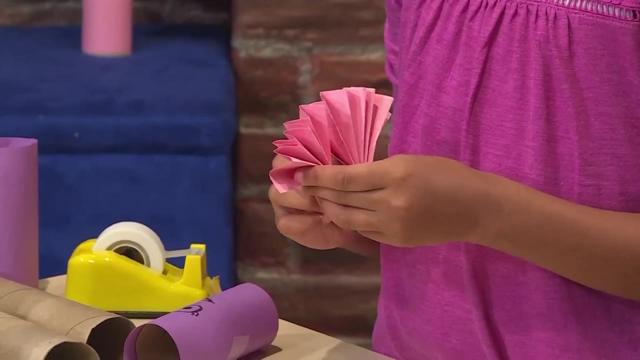 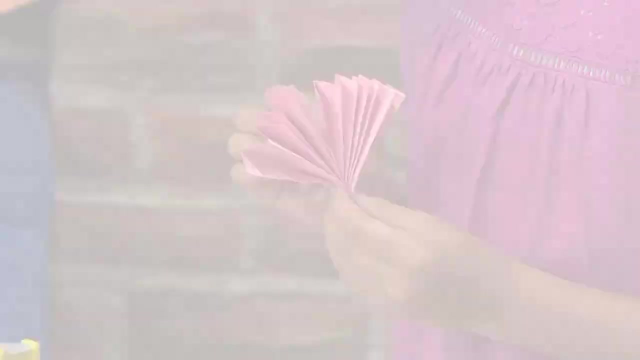 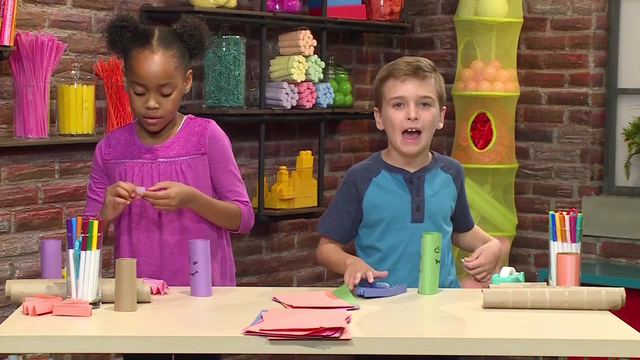 Once you have your fan, it will look like this: There, I made one. Then you fold your fan in half. Then you're going to tape the inside of the wing together. There, I have a wing, So do I. Then your wings get taped onto your bat. 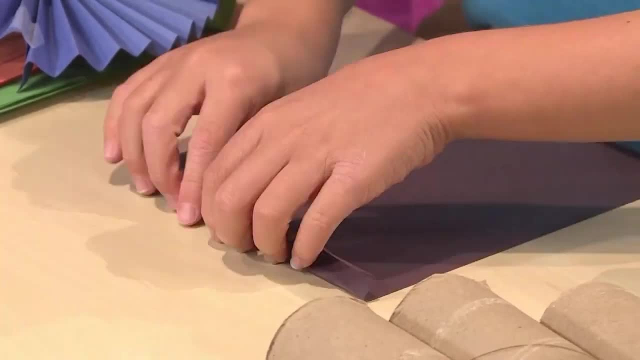 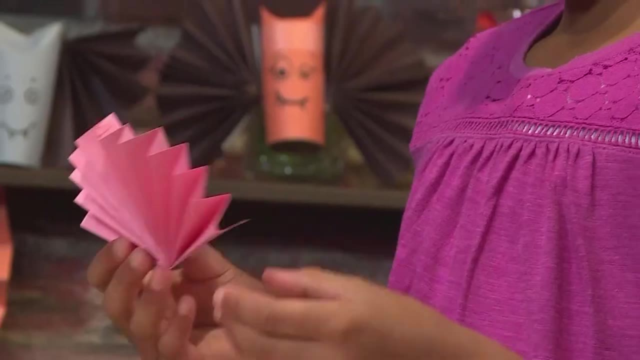 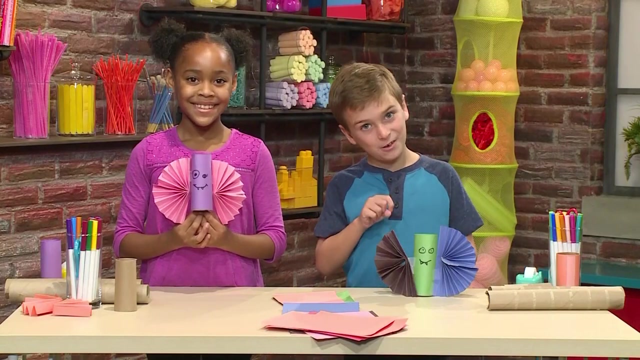 Then you add another wing to the other side. There I'm done. These bats might be really good for a Halloween party. I made my other wing, I got my other wing on and it's balancing. One last step: The ears. 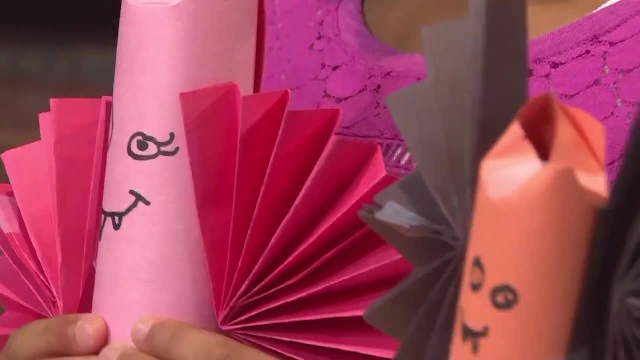 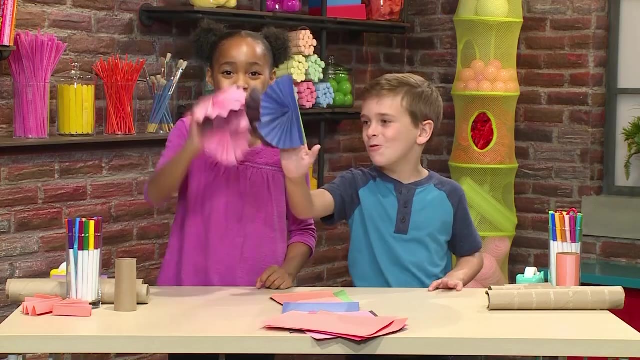 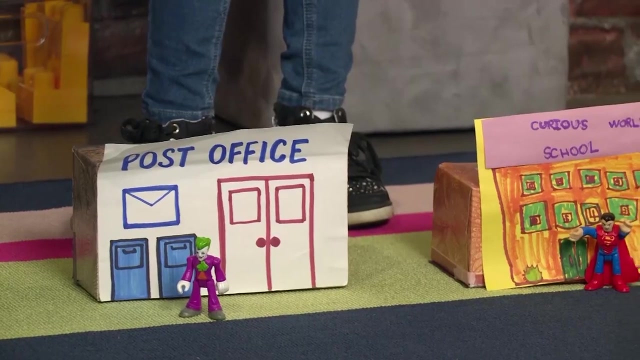 Just press down the middle of your toilet paper tube. That's the best part about Halloween: You just make stuff up And that's how you make a Halloween bat. Oooooooo, Hero City, Hero City. Let's make a small city for our action figures. 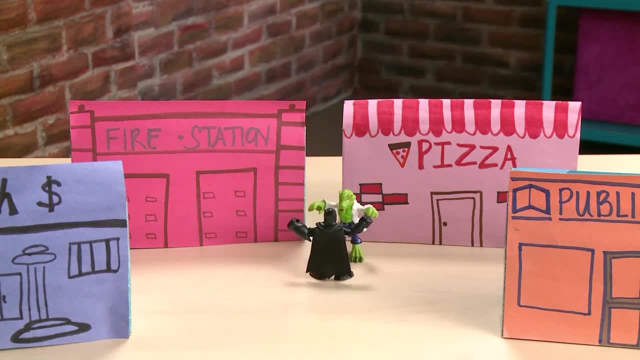 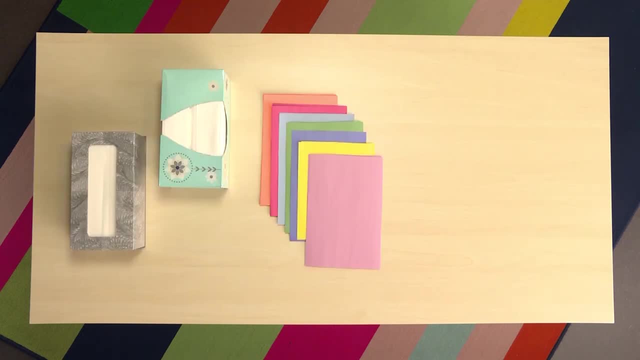 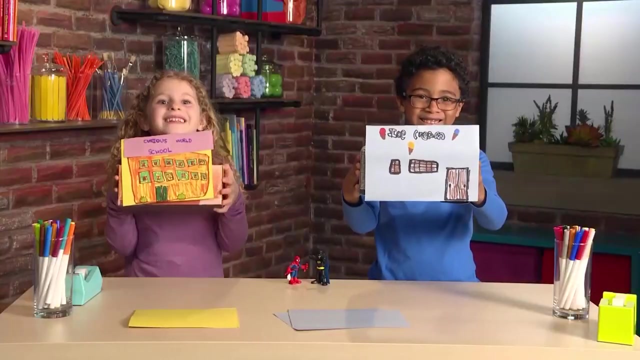 Pow Woosh, Pow, Woosh Pang. The things you need to build a hero city are Tissue boxes, Construction paper Markers And tape Tissue boxes. The tissue boxes will be our buildings Construction paper. 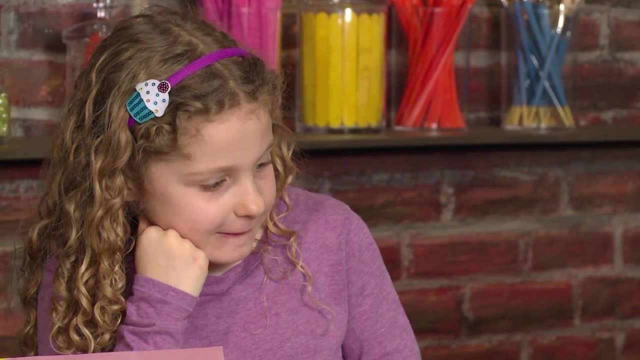 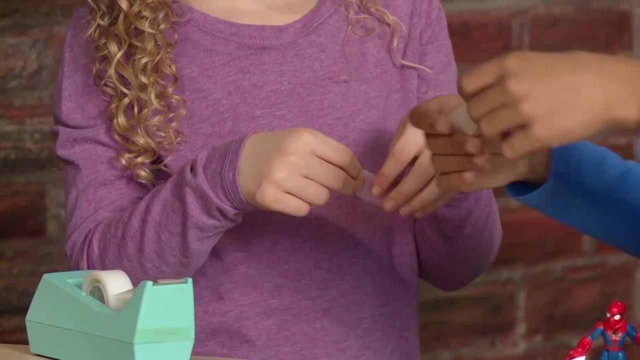 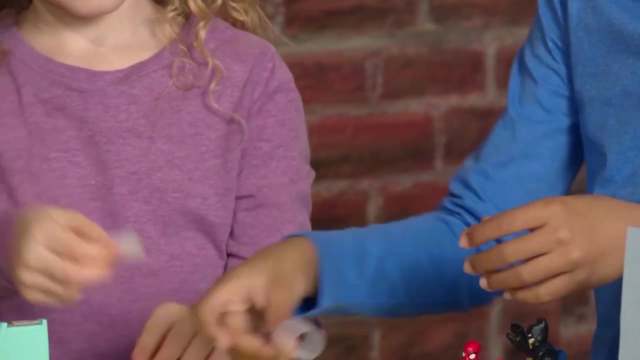 Draw the buildings on the construction paper. Hmm, what should we draw? I'm making an ice cream parlor. I'm drawing a school. I'm making a tape loop. To make a tape loop, you have to take the sticky part and put it on the sticky part. 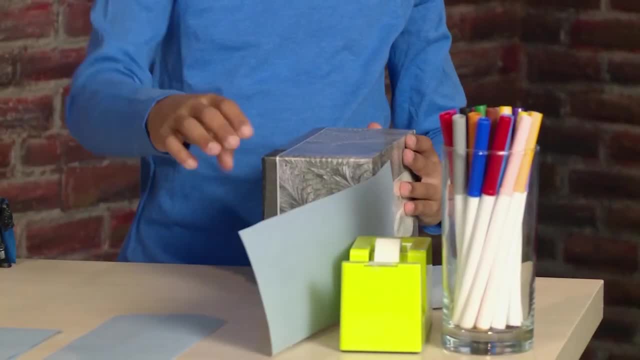 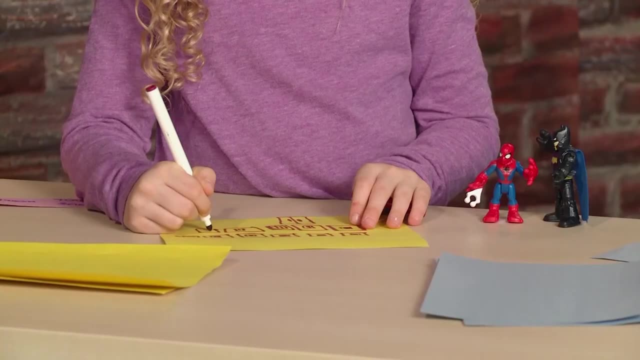 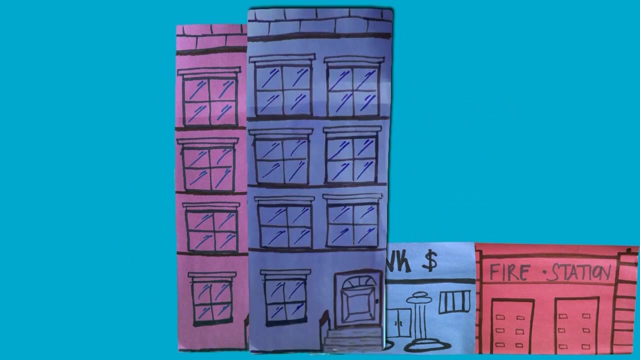 Ta-da: Assemble the building. Take the construction paper on the tissue box, Press the paper onto the tissue box. Let's draw all our different buildings: Skyscraper, Fire station, Bank, An apartment building, Post office, Pizza parlor. 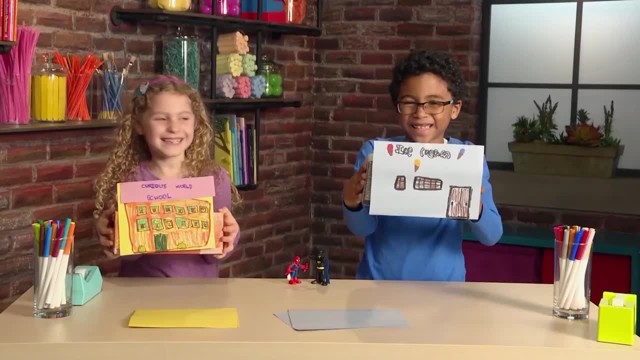 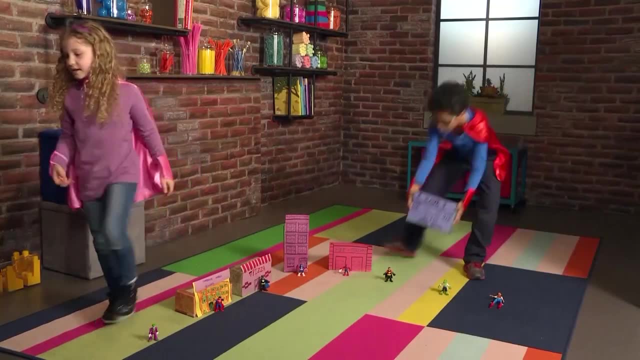 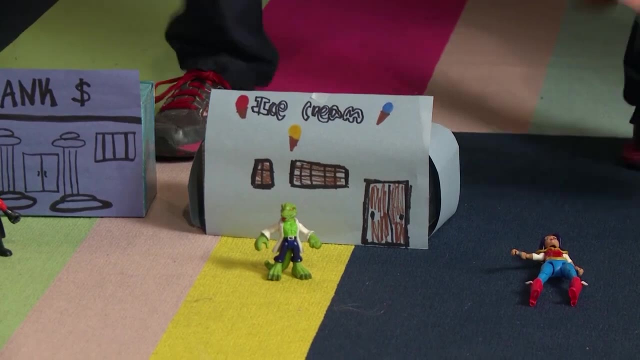 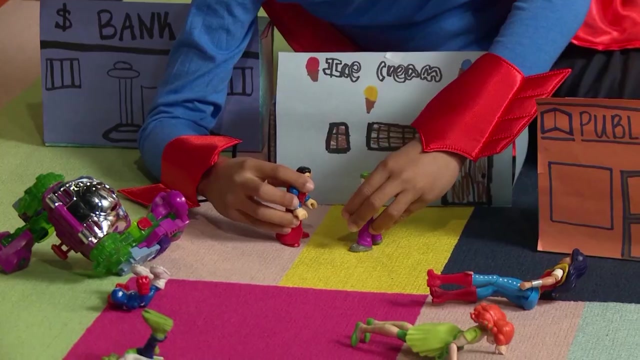 Now you have your buildings, Hero City, here we come. Time to play. Someone's eating all the ice cream. Help, Pow, Woosh Pow. We'll save all the ice cream in Hero City. Yes, We saved the ice cream. 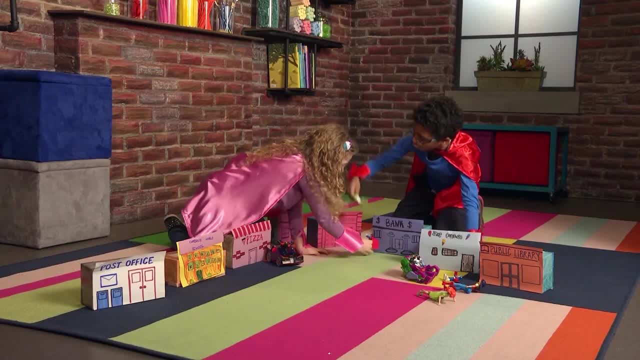 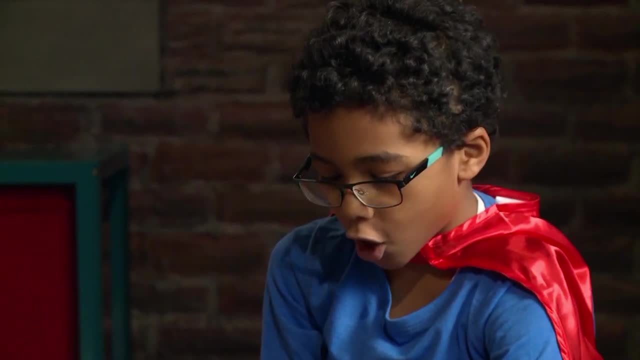 It's time to sneak into the bank, Not so fast. Oh no, The villain. We have to protect everyone. I'm on a mission, Let's go. Bing bing Wee, Bing bing, Wee, Bing bing Wee. 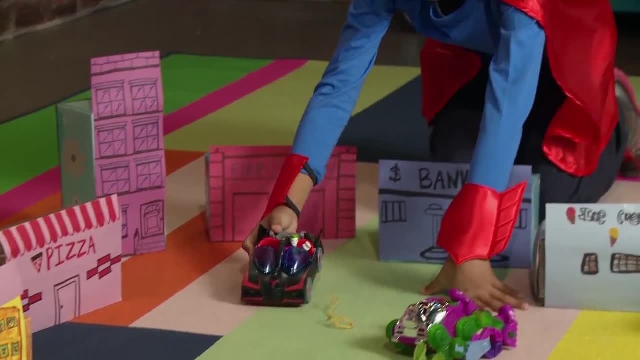 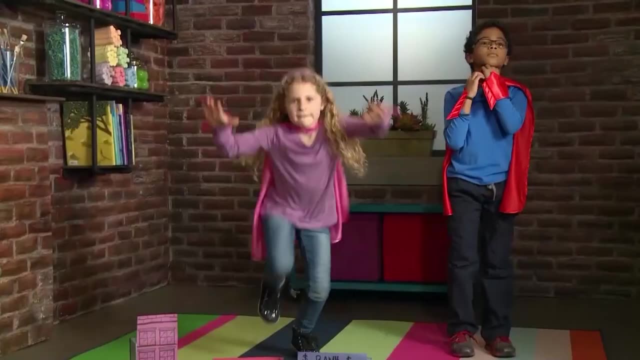 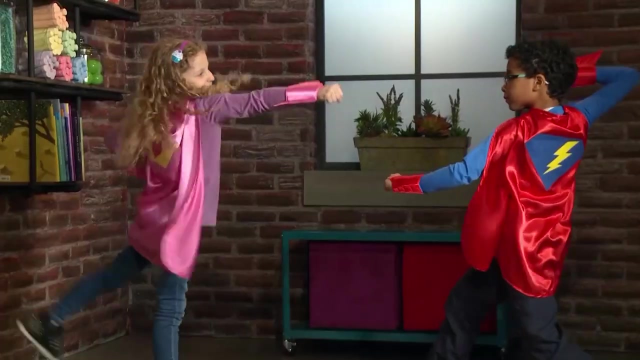 Let's hop in the car. Let's go Up, up and away. Pow Bang, Crash Bam. Here we go. Time to fly Hero City. Hero City is safe again Until tomorrow. How to make your own city. 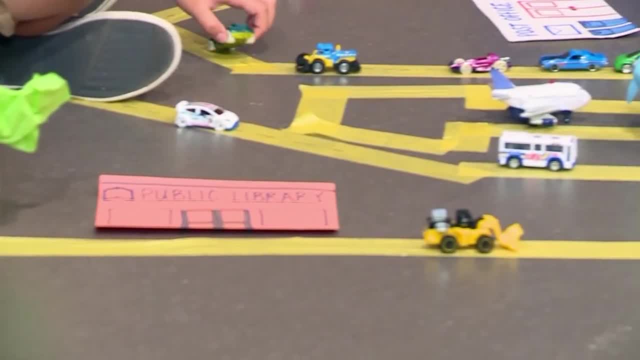 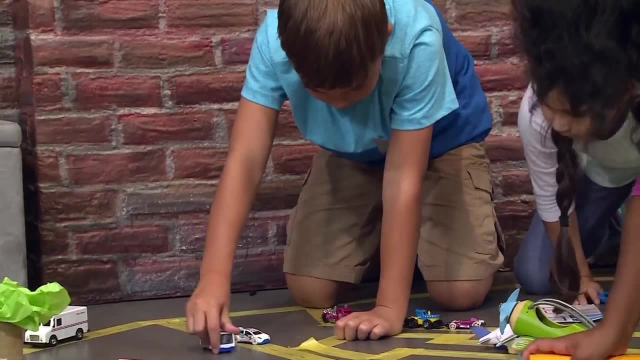 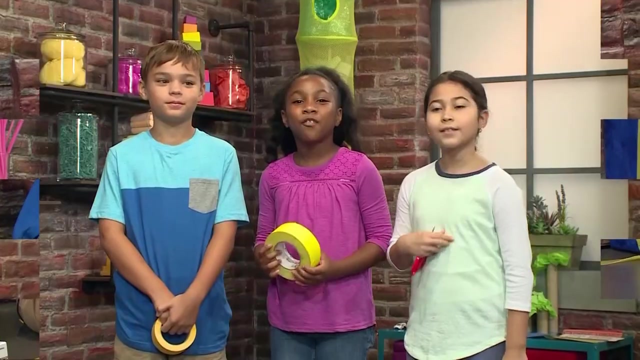 Vroom, Vroom. We made our own city. today We're playing with cars and roads. We're going to show you how to do it so you can play too. Beep, Beep, Beep. The first thing that you need to make your own city is masking tape.